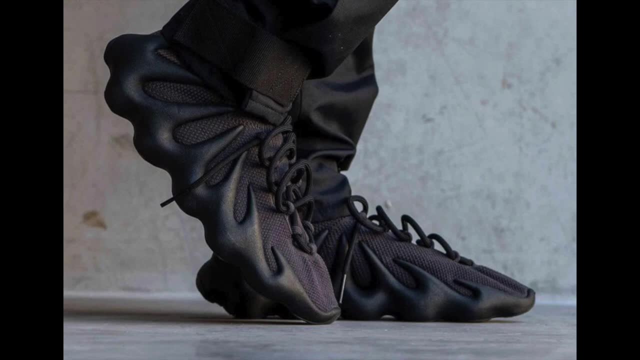 this right here fire. So the Yeezy 450 Dark Slate is set to release on June 25th 2021, and this is a Friday. Now, as we take a closer look into the shoe we're going to dive into that midsole man, I mean. 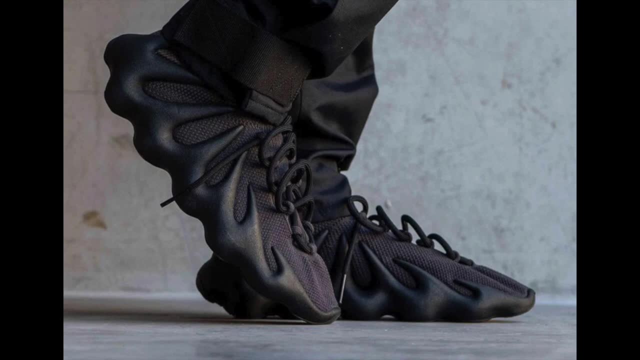 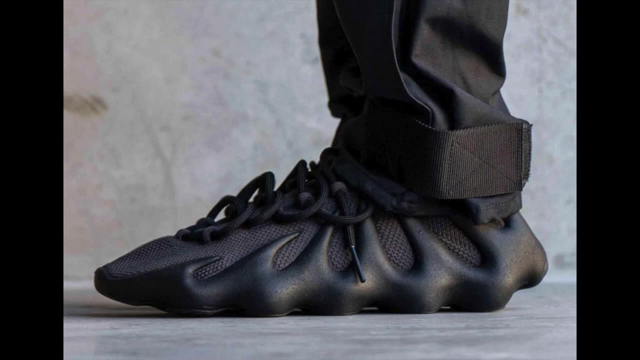 it just looks like a. it just reminds me of that. what's the name of that Spider-Man character, Venom? It just reminds me of these shoes, I don't know. I just see that all dark slate. That is a beautiful pitch dark. Look at the way the midsole just eats into the upper of the shoe. That's why. 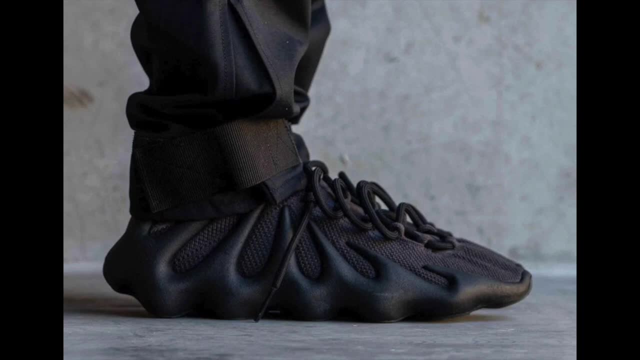 I like about this shoe is this shoe just gives me a futuristic, real grimy, like evil villain type of vibe. You know what I'm saying. Like y'all might not agree with me, but y'all definitely can see where I'm coming from If you really take a deep look into like just the silhouette itself. 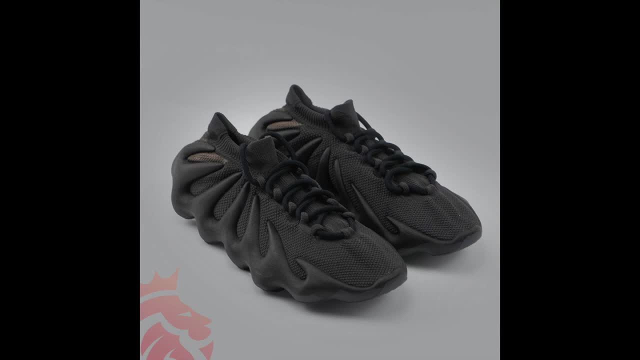 it looks very like you know just- I don't know- very reminiscent to a scary movie character. for some reason It reminds me of some teeth. but as we get into the upper it's just going to be a darker upper and a darker lower. Um now, like I said, guys, 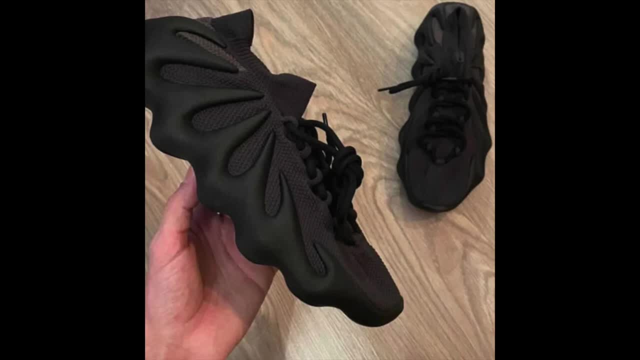 is set to release on the 25th of June. Um, the cloud white was the first one And this is the second colorway. Um, let me know what you guys think. down below this shoe right here is definitely going to be something dope And, as I told y'all before, I am going to try to get the shoe I do. 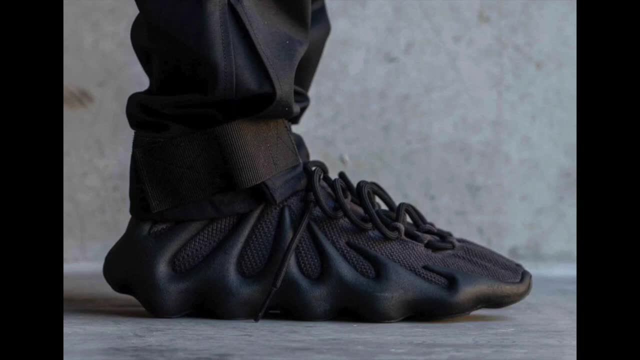 not have the shoe in my possession and I've never seen one of these before, So I'm definitely interested in getting one of these and my possession and do a review on these. So, like I said, guys, what do you think of this? This is a cop, This is a drop. Let me know now. impact wise. 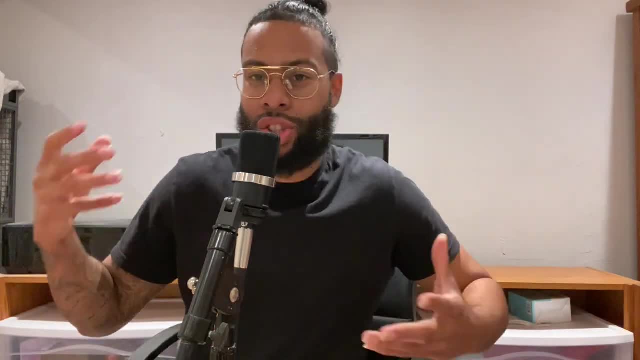 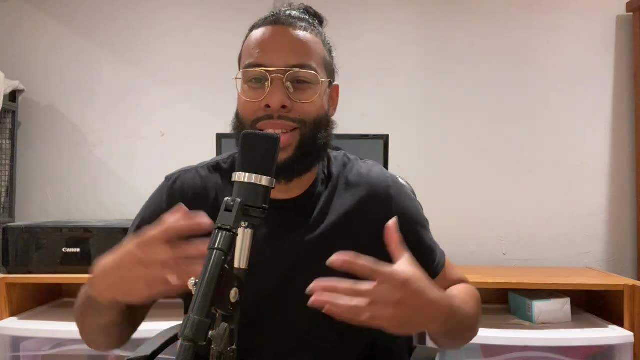 guys, when it comes to this shoe, um, not, not too much noise, I know. I think when the shoe first came out, a lot of people were jumping the broom like, Oh, this is cool, This is crazy. And it was like, almost like shock value. 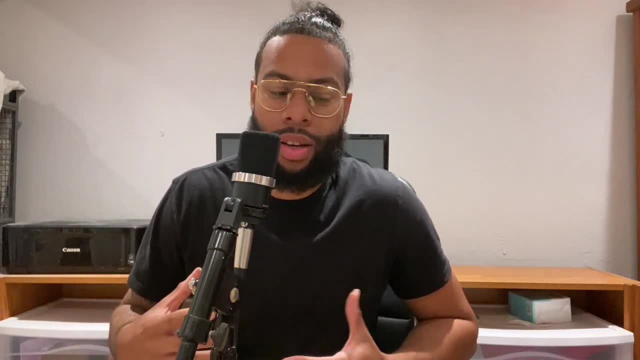 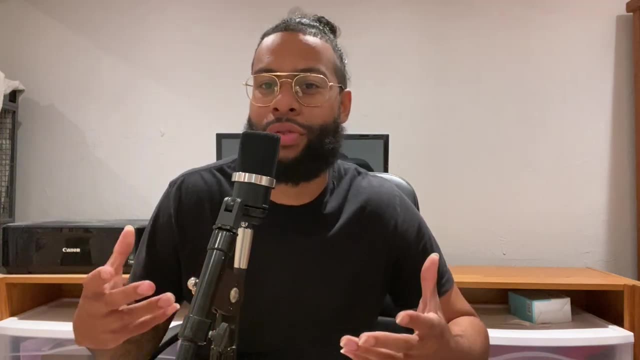 Like a lot of Kanye shoes are just shock value. It just becomes I don't know like almost not, not like a, not like an internet sensation or internet troll thing, because it looks so different and it's not what people are used to. But, like I said, that's why I enjoy the shoe, because it's 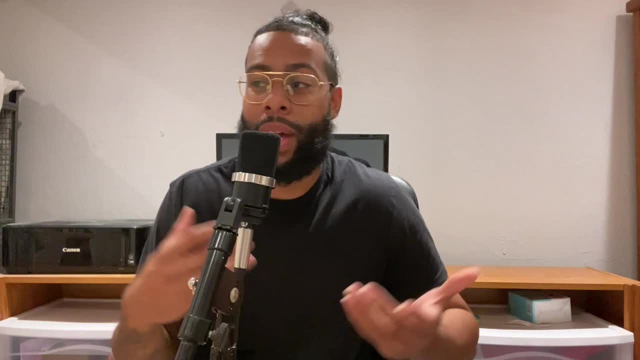 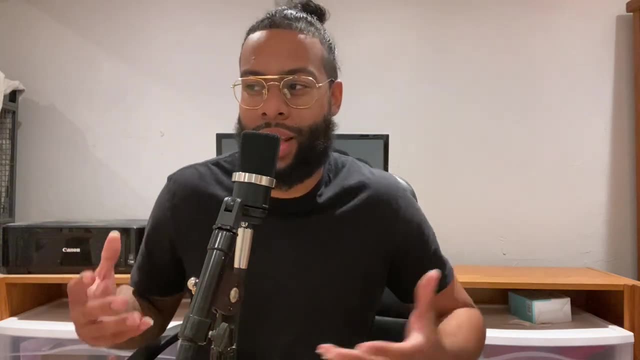 different. It's not the same silhouette that we've been seeing for a long time, It's. it's just different And I can't agree. Uh, and I can't disagree if someone says they don't like it or agree it says something, because everybody's going to have their own opinion at the end of the day. 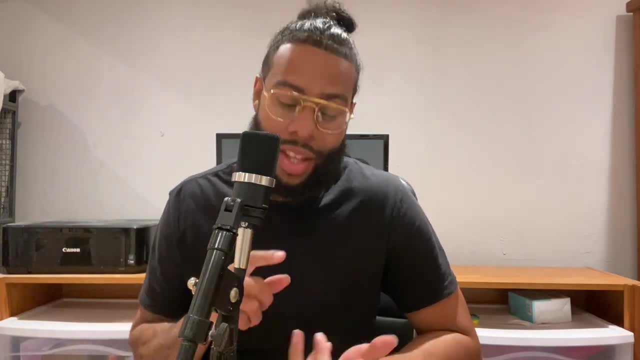 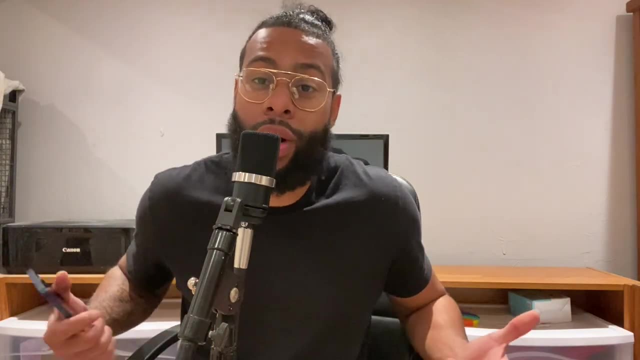 And this shoe to me is definitely a cop. I do want to get my hands on either the cloud whites or these ones right The dark slates, because I just never seen them, And I want to get these in my possession to see what they look like. And, as we know also guys, you know, usually all black. 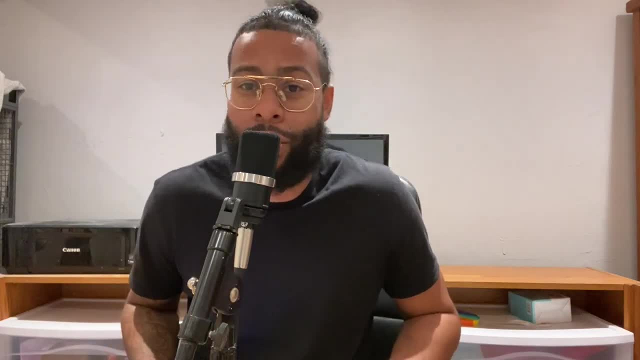 Yeezys are hit. So you know: three fifties bread, three fifties a nice all black. I mean this, this is something about that all black color that just hits Now when it comes to. 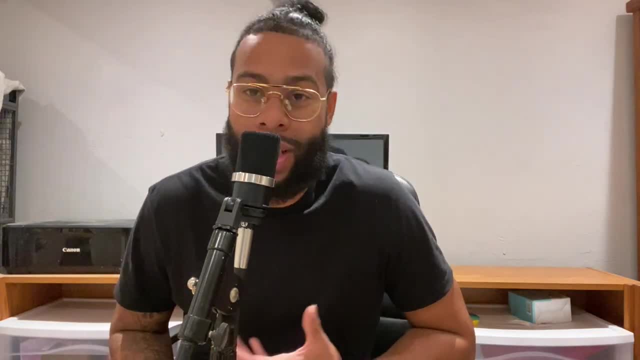 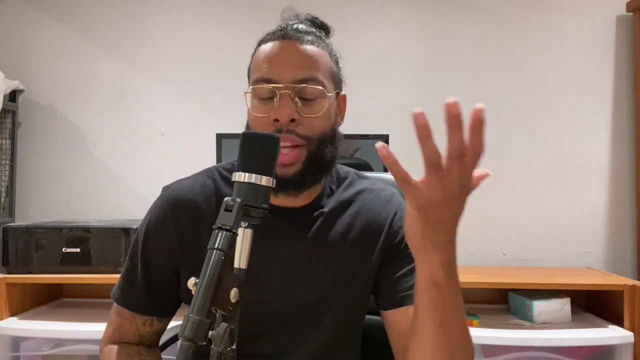 where to buy the shoe. we do have the usual suspects, as always: Yeezy supply, check your sneakers and stuff app. Make sure you follow a lot of these bodega spots, expressions, a lot of places that do raffles with shoes. As always, you just want to be up on who. 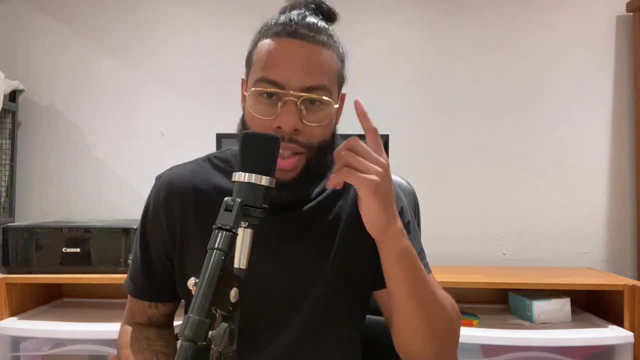 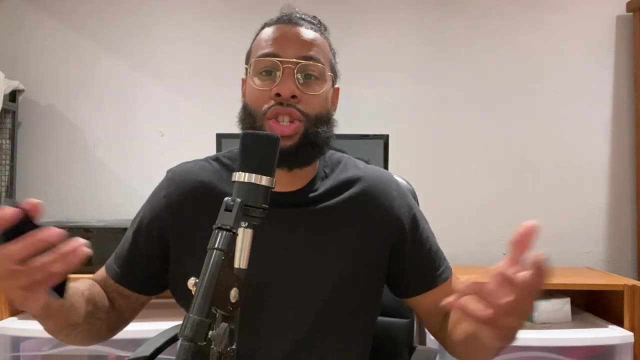 has the shoe. A lot of places will have the shoe, and you just got to be smart enough to know which spots to have and which spots to follow, because you definitely want to be following the right spots, just in case these shoes do drop somewhere. You have access Now. these are set to be released. on June 25th for retail price of $200.. Now let's just get into some reset value. So I pulled up GOAT. right now I'm looking at the average price of the Yeezy 450 cloud white. I'm looking at the Yeezy cloud white right now on GOAT. It's going for about $436 and upwards towards the $500,. 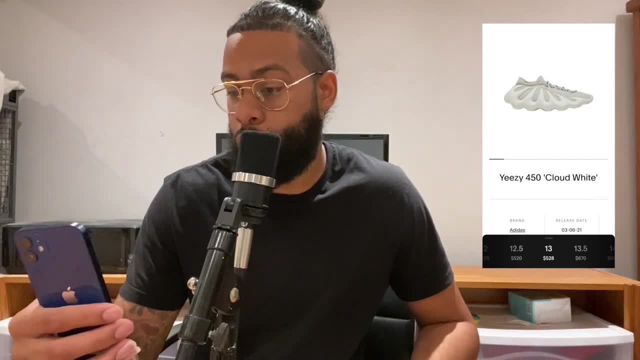 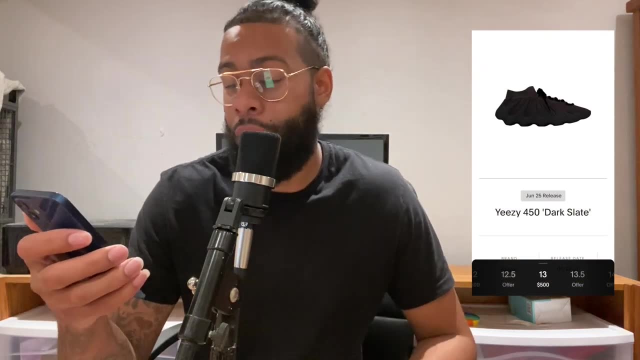 $600 marks. You know what I'm saying- Depending on what size you have. you know well: $400, $500, $600, depending on the size. Now, right now, I already see the Yeezy 450 dark slates going for a price of about $500 plus. 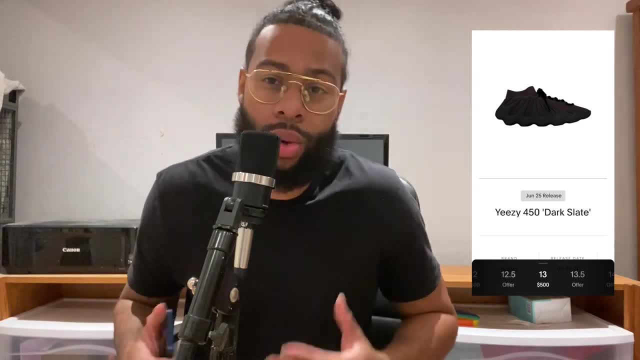 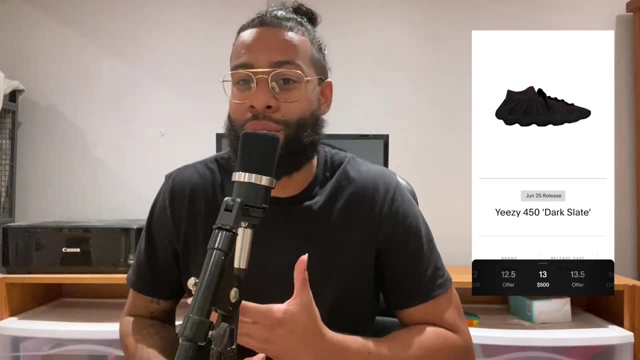 Now, this is before release. So once I expect the shoe to release, I do expect the price to drop down a little bit. but just in general the 450s are not a bad when it comes to resellers. So resellers out there, if you're interested in reselling the shoe, this might be a shoe you 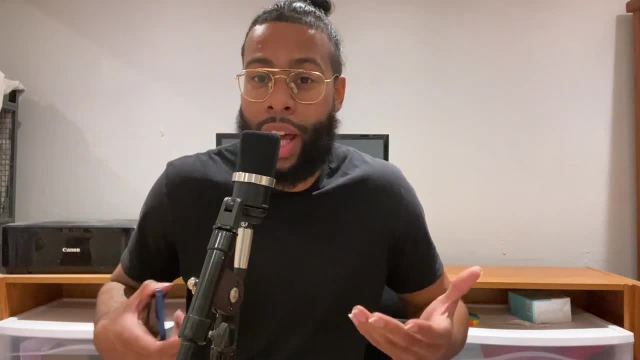 definitely want to grab. Like I said, it's, it's really nice shoe And and if you want to rock it you can rock it. But if you want to flip it to make some money you definitely can make a little. 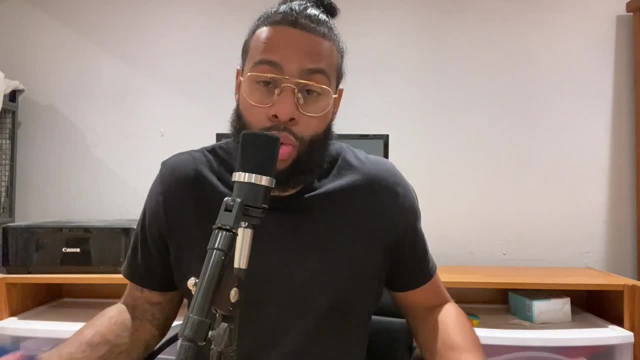 bit of money on the shoe. maybe two to $300 you can make if you go ahead and cop the shoe. So, with that being said, guys, like I said, I do apologize, for you know what's going on right now.